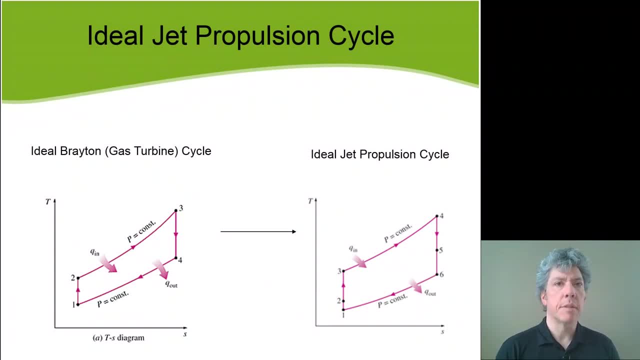 Another cycle to study is the ideal jet propulsion cycle. It's based on the Brayton cycle because in an ideal jet propulsion cycle there is a compressor and a turbine, much like in a regular gas turbine engine. So you'll notice that the TS diagram for the jet propulsion 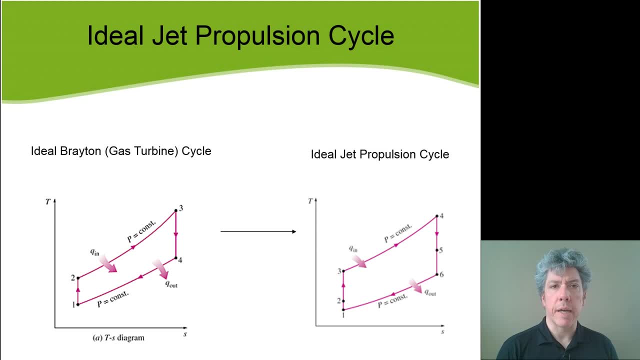 cycle on the right looks a lot like the one on the left, that is, for a gas turbine cycle or Brayton cycle without regeneration. Now you'll notice that on the right hand side the ideal jet propulsion cycle has a couple of intermediate states during the compression. 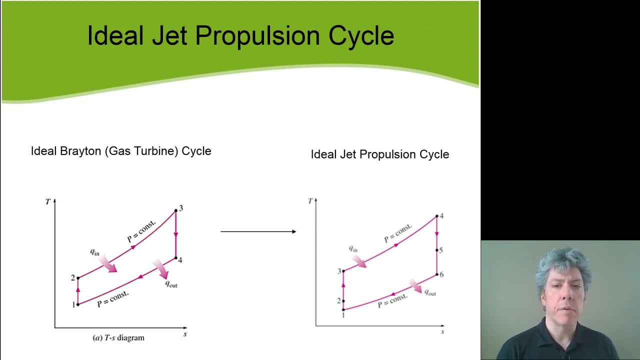 process: on the left, the vertical line, on the left, state one, two, three and on the right, during the expansion process in the turbine from state four to five to six. Now, why do we have state one to two in the gas turbine cycle? being all of it and in the ideal, 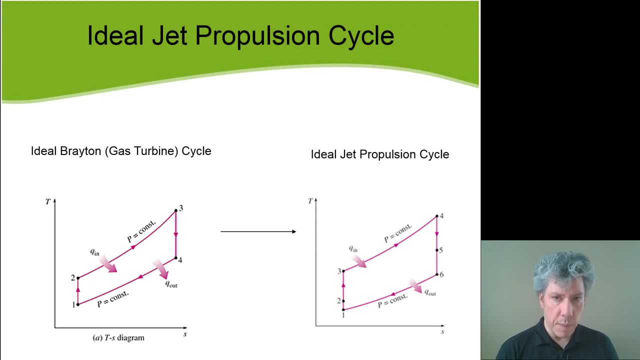 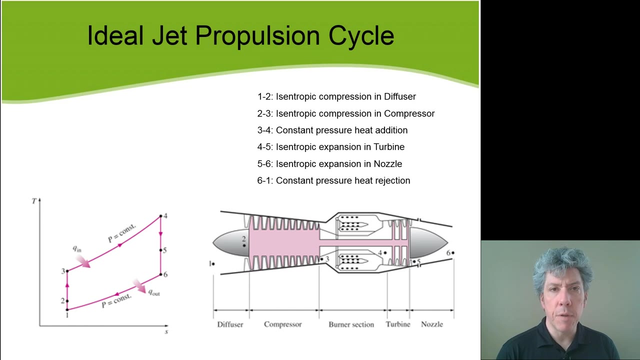 jet propulsion cycle, we've got three states being all of the isentropic compression process. Why indeed? Well, the reason is because the jet engine works a little bit differently than the simple gas turbine. The key difference is the addition of a diffuser on the front of the engine and 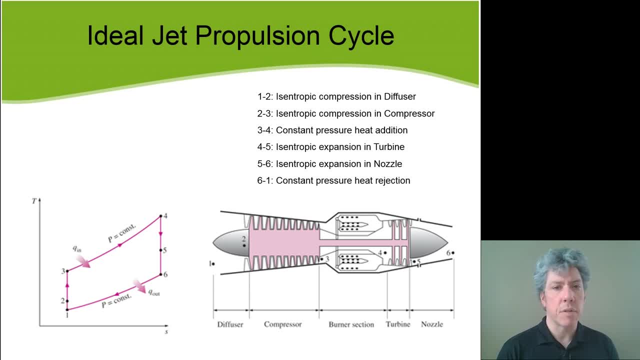 a nozzle on the back end. Now, if you look at these and consider the cross sectional areas, the diffuser looks more like a nozzle than the nozzle looks more like a diffuser, But the idea is that the entrance to the diffuser is smaller than the exit of the diffuser. 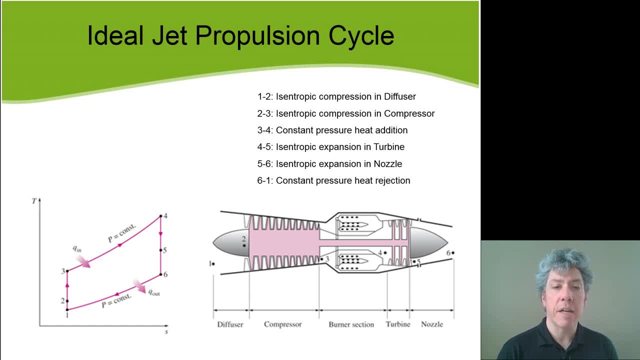 So, moving from state one to state two, It is moving through the diffuser, so the area of state two is greater than the area of state one, even though this graphic doesn't really illustrate it properly. So what happens in this engine is very much like what happens in the gas turbine engine. 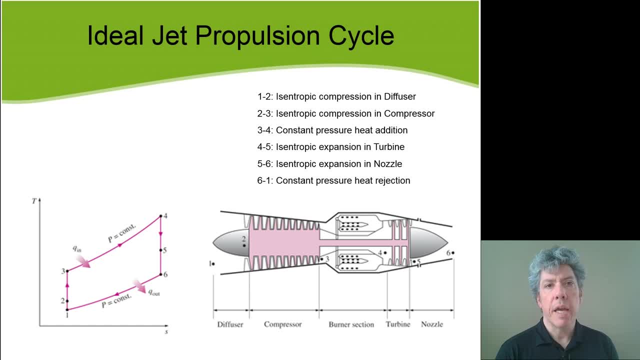 except that there's the diffuser at the beginning. So state one to state two is an isentropic compression in the diffuser. at least ideally Understand this is the ideal jet propulsion cycle. No, diffuser is going to be isentropic, But again, hopefully we can get close by designing. 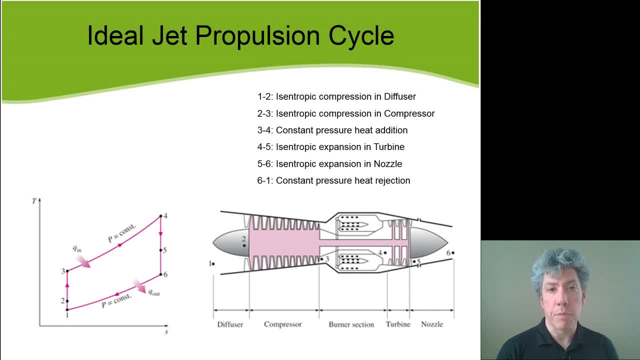 it well, From state two to state three is compression in a compressor, and so that is again ideally isentropic compression. State three to state four is very much like what would happen in a regular gas turbine engine, where fuel is added to very hot air so that it burns in. 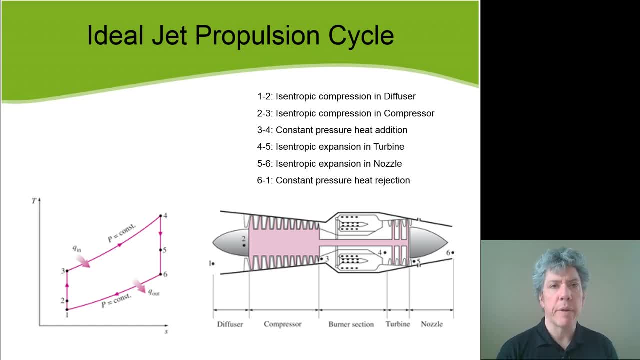 a continuous fashion, And one key thing to note about gas turbine engines and jet engines and so forth is that anytime you have a compressor wheel in a turbine, you really want it to operate continuously In the gas. you can put in a charge and light it up and do more of a batch process of burning. 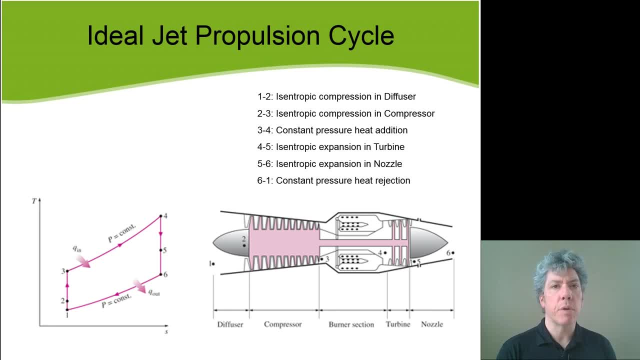 fuel. but in these bladed type engines, where you have compressor wheels and turbine wheels, you typically have a more continuous burn, And I really am interested in this type of engine because it's much easier to tightly control a continuous process than a batch process. So anyway, moving on from state three to state four is the burner section, and this is just. 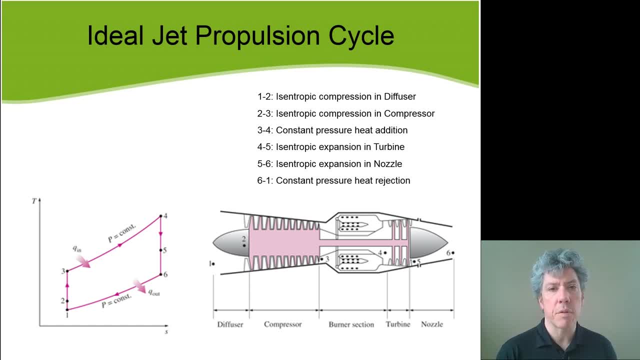 an open section. So the pressure is constant from state three to state four and this is where, of course, fuel is added and burned. so this is our constant pressure heat addition process. And then, going from state four to state five, is the move through the turbine, where the 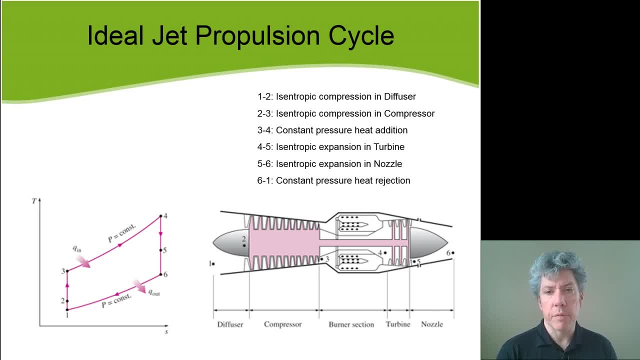 hot gases expand in the turbine, going down to reduced pressure, giving up energy along the way. Of course, their enthalpy decreases because it's both the thermal energy and the flow energy, in other words the enthalpy, that is given up from the fluid. 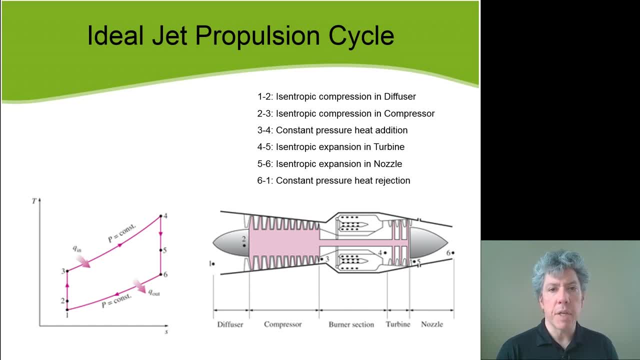 In order to drive the turbine blades, And then from state six to state one- I'm sorry, pardon me- from state five to state six. at the end of the engine in the nozzle is further expansion, isentropic expansion in the nozzle, and then from state six to state one is constant pressure heat rejection. 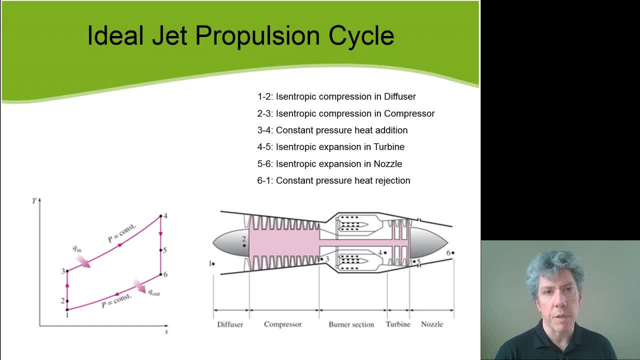 Now that constant pressure heat rejection would occur in the atmosphere and of course, as usual, we'll replace that process with a heat exchanger. essentially, that takes the hot air out the back of the engine And then puts it back in. So anyway, this is the jet engine cycle and there's a couple of important things to note. 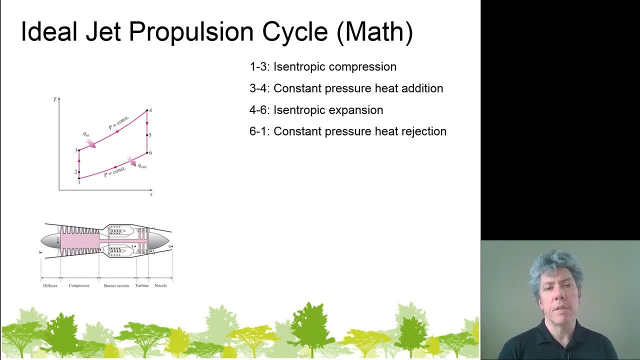 First of all, if you look at the cycle diagram, you'd realize that really state one all the way to state three are related isentropically, And so for the very simple ideal jet propulsion cycle, all you really need is an isentropic relationship between states one, two and three. 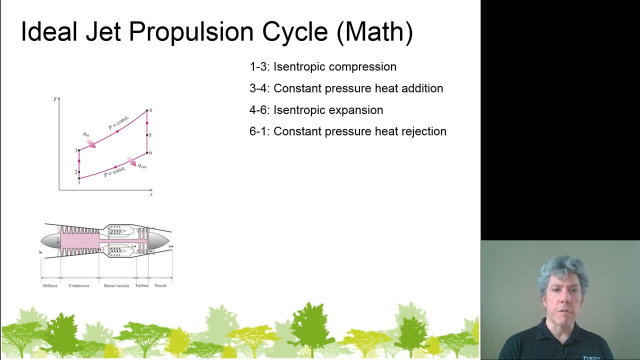 And, depending on the problem, you just use whichever cycle, Whichever states are convenient. From state three to state four is constant pressure, heat rejection, Then four to six is isentropic expansion. Another move through three states, Three states that are all isentropically related. 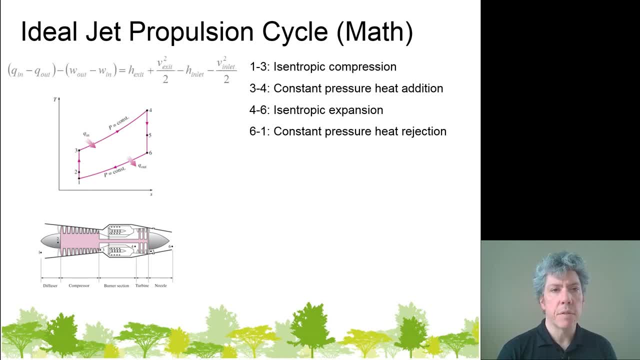 And the six to one is constant pressure, heat rejection. Now there's, of course, an energy balance that we can consider in all of these sections of the jet engine, And that energy balance has to include enthalpies as well as velocities, Because the purpose of a jet engine like this is not so much to generate work output. 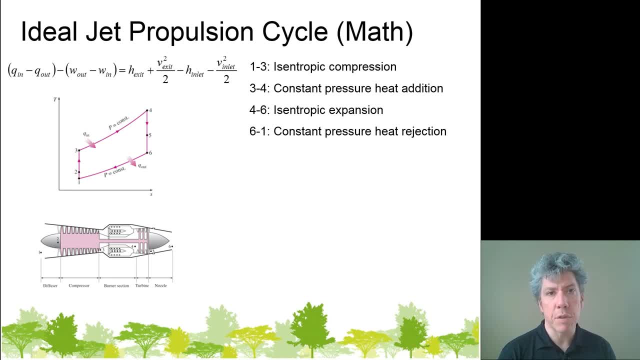 As a matter of fact, the majority of the work produced by the turbine is used to drive the compressor. Now, in a real jet engine or a real plane, yes, some work is extracted to drive things like hydraulic pumps for controlling control surfaces or moving control surfaces on the wings. 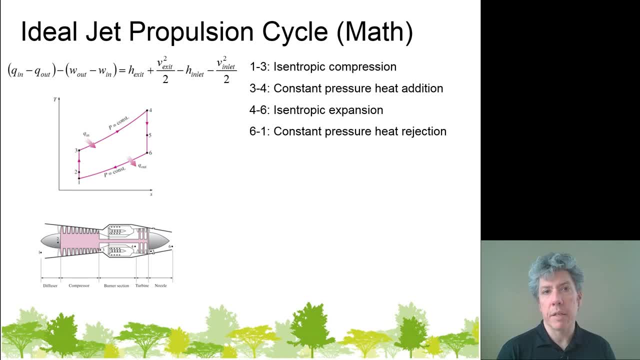 Some power is extracted for generating electricity. You know Cabin electronics and lights and so forth. Some energy is extracted. I'm not sure if it's off the engine itself, but some energy is certainly extracted and used to drive air conditioning and things of that nature. 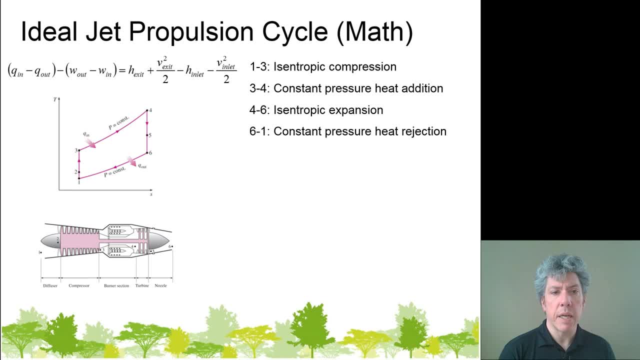 So there's more to it than what you see here. But for all practical purposes there's a relationship between the output work of the turbine and the input work to the compressor, And we'll get to that in just a second. For right now, just understand that you can write an isentropic equation. 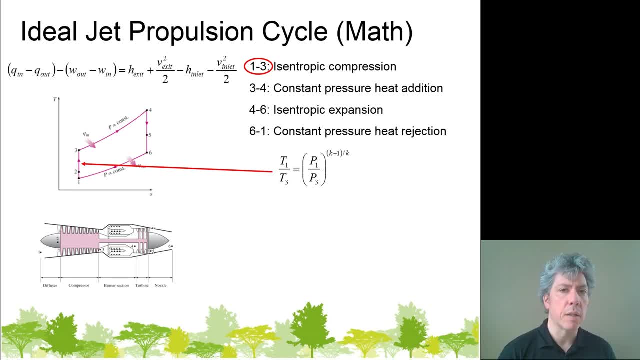 You can use a state 1,, 2,, 3, interchange them however you want. They're all isentropically related. in the ideal jet propulsion cycle During the heat addition process in the burner- the best equation- there is an energy balance that notes that any thermal energy that comes in via heat increases the enthalpy of the 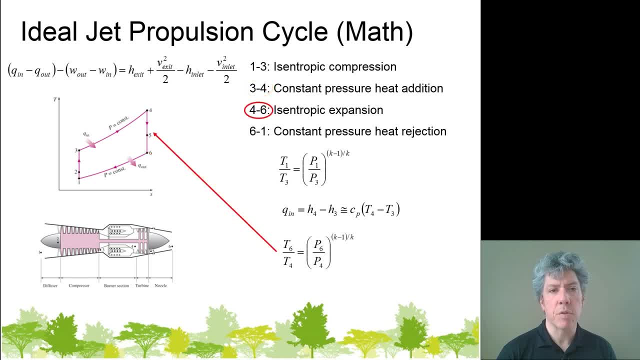 air flowing through that section. And of course an isentropic relationship is appropriate for the last three states. It's going from the inlet of the turbine all the way through to the exit of the nozzle, And then an energy balance for the heat loss in the atmosphere is an appropriate equation. 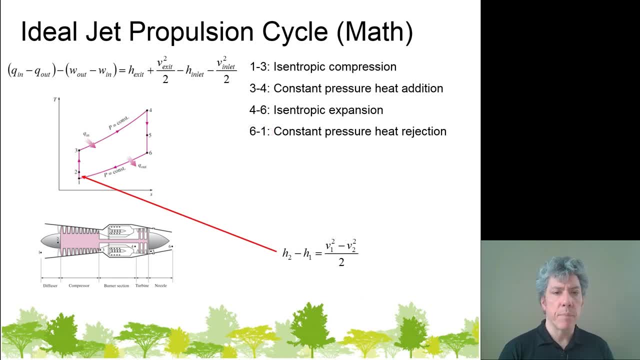 as well. Now, all of that's well and good and you should use them, but there's a couple of other equations you really need that are unique to the jet propulsion cycle. One of them is the energy balance around the diffuser itself. So, while there is an isentropic relationship, 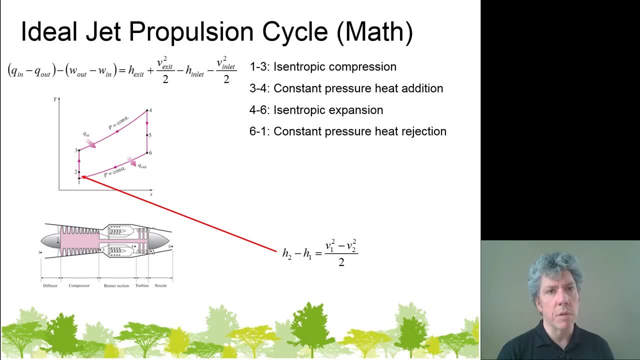 Between states 1 and 2 across the diffuser. The energy balance here will also come in pretty handy, And so the enthalpy change between the two states of the air is just driven by the kinetic energy. In other words, there's excess kinetic energy coming into the diffuser, but since the flow 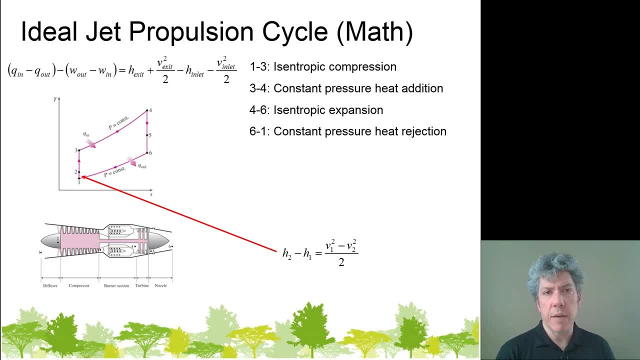 area increases and the flow slows down. that energy can't be destroyed, and so what happens is that kinetic energy is changed into enthalpy flow energy and thermal energy, in other words, And so that equation is very useful. Often, we will neglect the exiting velocity of the air coming out of the diffuser and going. 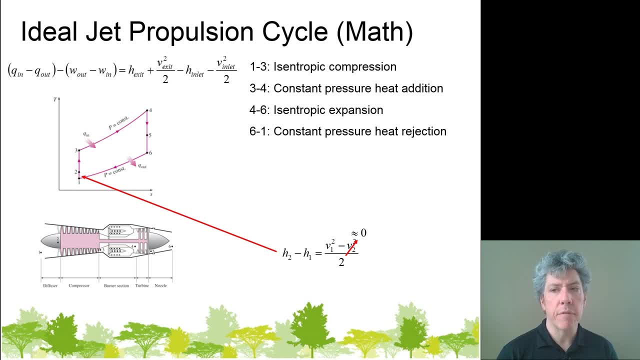 into the compressor, And so a lot of times this energy balance will have the kinetic energy term- the velocity at the exit of the diffuser- just crossed off. Similarly, an energy balance is particularly useful for the nozzle at the back end of the engine, And what it does, of course, is actually a very important function. the outlet gases at state. 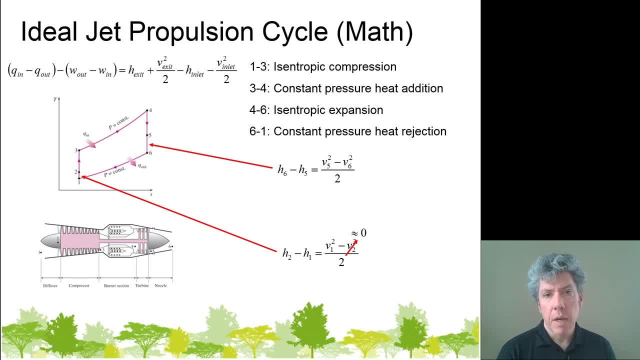 5. The nozzle is a very significant amount of energy in them. As a matter of fact, that energy is so great. some of it can be converted and used to generate kinetic energy, because really the purpose of a jet engine is to generate kinetic energy. 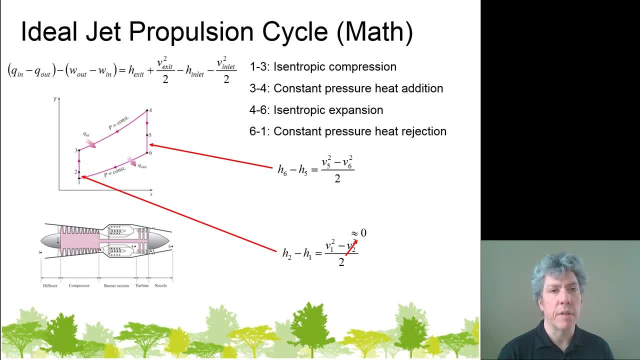 It's to push air, essentially out the back of the engine so hard and so fast that the engine is pushed forward and therefore the craft that the engine is attached to is also pushed forward. Now again with this nozzle, a lot of times we will assume that the kinetic energy, that's 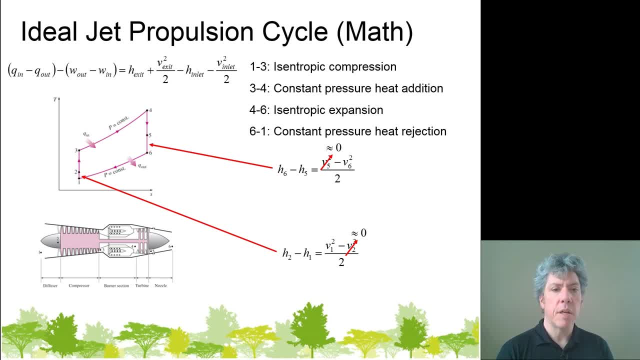 coming out of the engine is actually the energy that's coming out of the engine, And so that's what we're going to do. So that's what we're going to do. So the kinetic energy of the air when it exits the turbine is so low that it's not 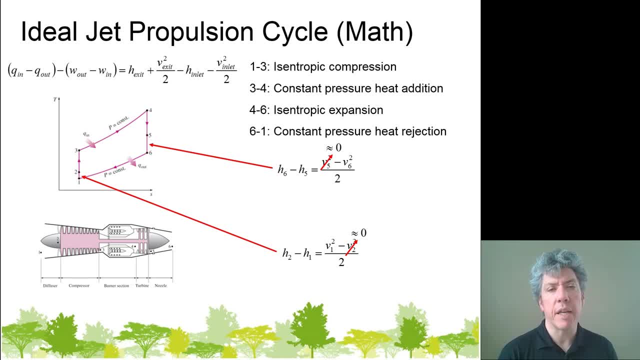 worth including in the equation, and that the kinetic energy at the exit is completely generated from the change in enthalpy. Now there's one more equation that is very important, and it is related to an energy balance as well between the turbine and the compressor. 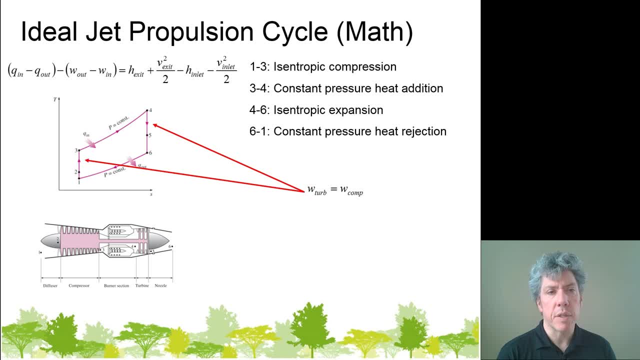 As I said before, most of the time we will assume- at least always in the ideal jet propulsion cycle- we will assume that the work produced by the turbine is consumed. It's consumed completely by the compressor. So you might look at this and say, well, that doesn't seem right, because so far all of these 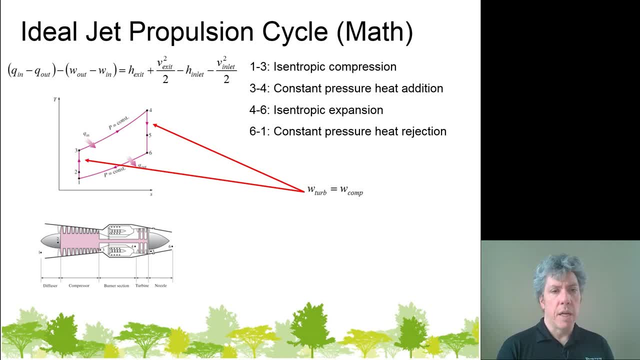 engines that we've dealt with have produced significant shaft work, And if this turbine blade is turning really fast, which is the case for these engines, it seems like there could be a lot of work available there. Well, it is, but it's all consumed. essentially, all of it is consumed by the compressor. 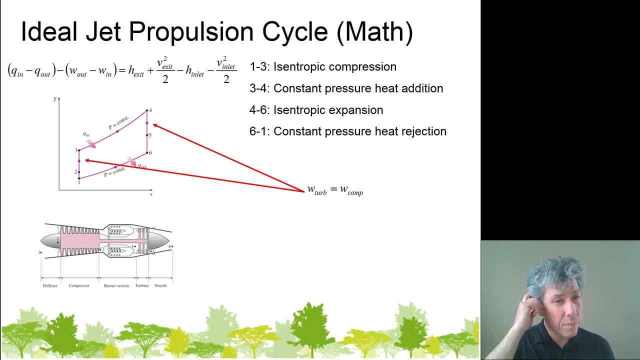 Because, remember, we're dealing with a gas and when we start talking about vapor power cycles, where the working fluid can move back and forth between the vapor and liquid phases, you'll see that the amount of energy required or the power that's required to recompress the liquid is a very small fraction of the power generated when the liquid that's been 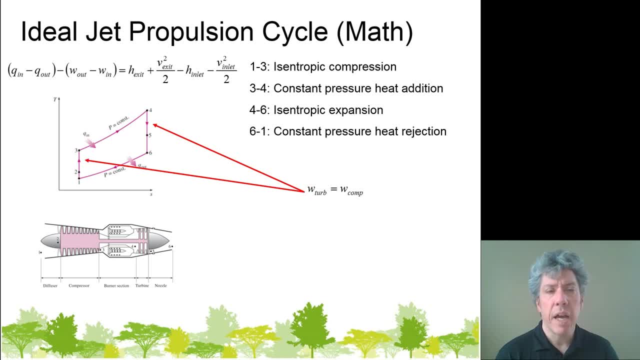 boiled off, goes into the vapor phase or the gas phase and then expands through the turbine. We don't have that luxury here. We're compressing a gas that has a relatively high specific volume, and so that takes a lot of work And, along the way, it doesn't take all of the energy. 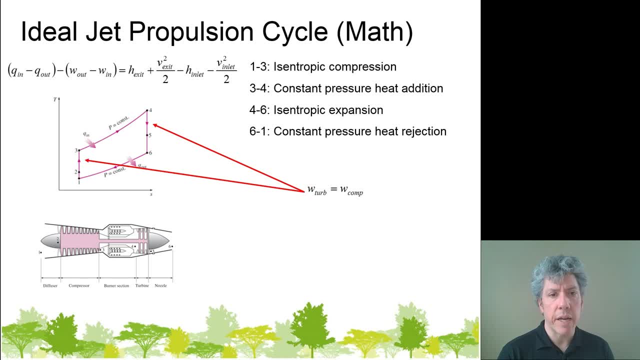 It takes a lot of work. The energy that we put into the air, the air leaving state five still has a significant amount of energy. So the main place where thrust is developed is in the nozzle of this engine, not by driving a propeller with these blades to pull the craft through the air. 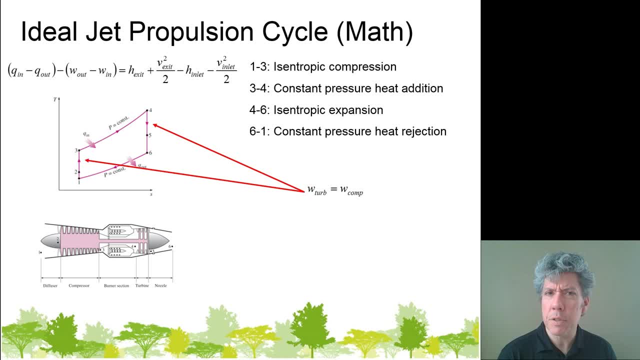 Now there are turbo prop. I think they're called turbo prop planes. turbo fan- no, turbo fan, I think, is the right term. We usually don't study those. They are in your book. if you want to read them, you're welcome to. 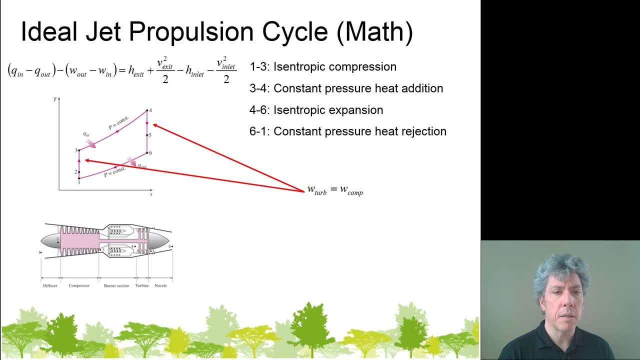 But turbo fan engines do include something that it's not exactly a propeller. basically, a turbo fan engine includes a fan on the front that pulls extra air through. So some of the work produced by the turbine is used to drive the compressor. Some of the other work produced by the turbine is used to drive the fan and then the fan. 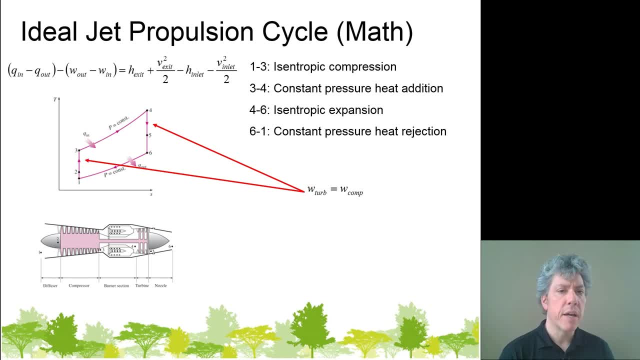 helps to pull air through and accelerate the air, pulling the craft through the air, And those are actually more efficient and more common than a strictly speaking jet in an engine. But anyway, here's what you need to know for the ideal jet cycle. If the work produced by the turbine is equal to the work consumed by the compressor, what? 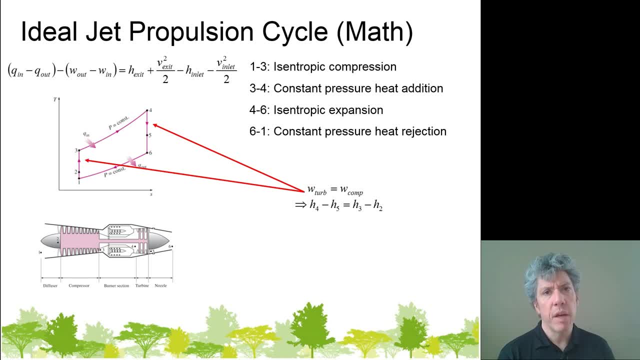 that means, then, is: since the mass flow rate through the compressor and the turbine are essentially equal, neglecting the fuel and the combustion products, since those two flows are essentially equal, then the enthalpy change across the compressor is equal to the enthalpy. 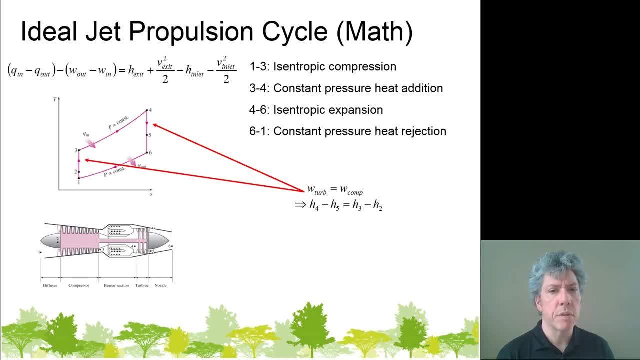 change across the turbine. That's a very important equation to know. It's based on the idea that all of the work produced by the turbine is consumed by the compressor, And so if we approximate these changes in enthalpy as Cp, delta, T, the heat capacity, 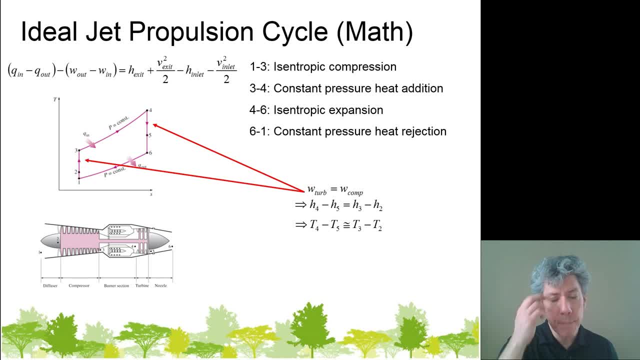 at constant pressure would cancel out, And here's a relationship. you should probably tab your book where this cycle diagram is located and you should probably write this equation and the others that I've already gone through on this slide next to the cycle diagram. If they're already in the book, you might just highlight them, but I would recommend 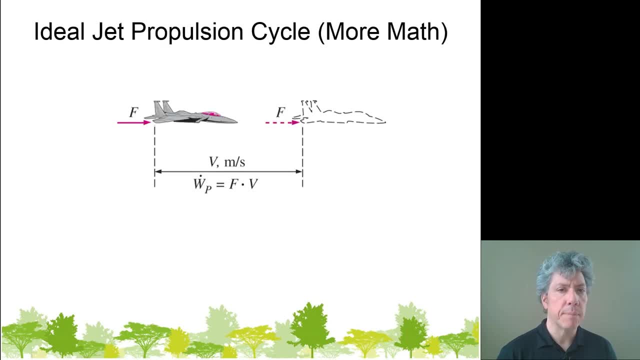 definitely tab it. The next thing we usually do is take 1-qa, q in over q out and calculate the efficiency and so on. but that doesn't work very well here, because really the goal of a jet engine is to produce thrust right. 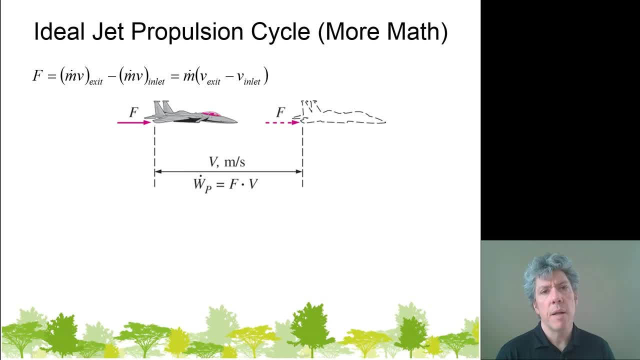 And so, really, what a jet engine does is it changes the momentum of the air before the engine to the momentum of the air after. In other words, it increases the momentum of the air. It changes the momentum of the air significantly, by a great amount. 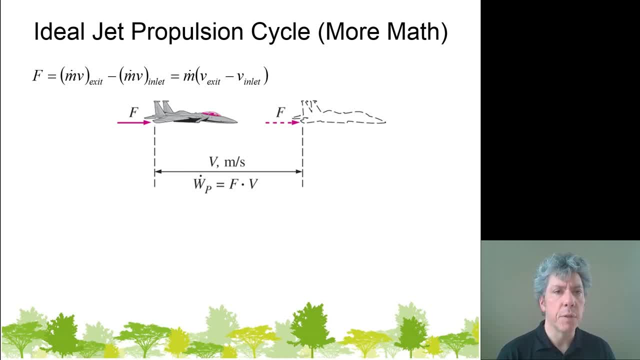 And if you remember from dynamics the way we calculate for fluids, we calculate thrust and things is, F equals the rate of change of momentum of that fluid. And so if you know the mass flow rate of the fluid through the engine and you know the 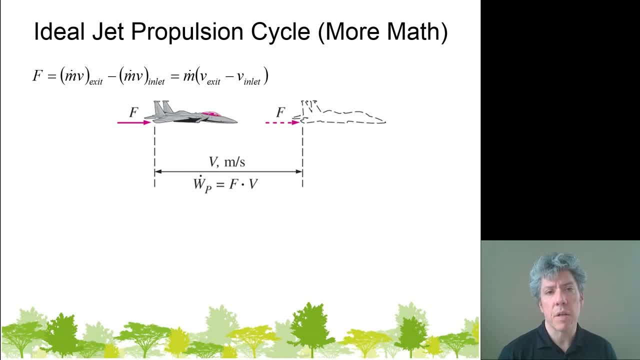 velocity at the exit of the engine and the velocity at the entrance of the engine of the air. you can calculate the thrust Now. The propulsive power is what we use to quantify the output of the engine, and so the propulsive power is equal to the thrust multiplied by the velocity of the aircraft, and this should.